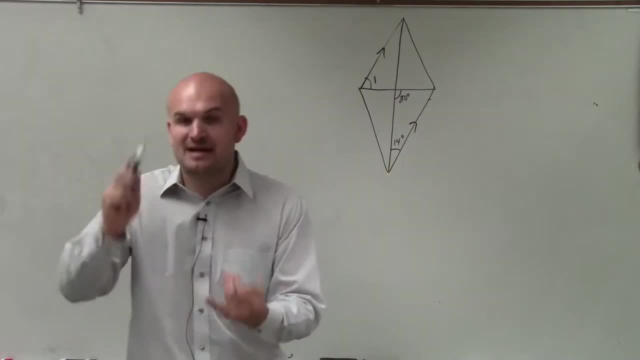 thinking of my angle, relationships alternate interior, alternate exterior, corresponding and same side interior, And I know it's kind of confusing because there's a lot of lines going on here, right? So if I'm looking at these parallel lines, I also see intersecting. 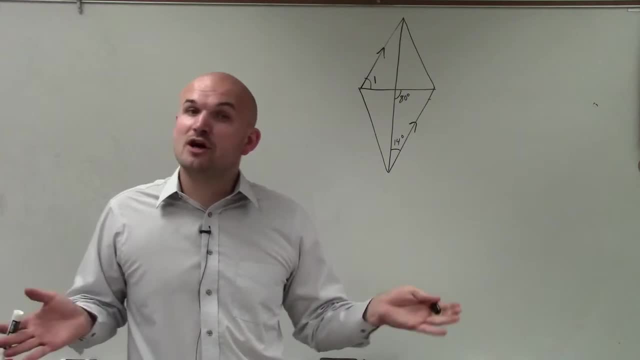 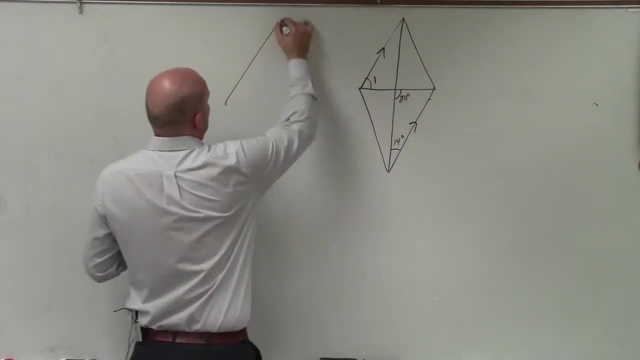 lines, which I should be careful, because intersecting lines also tell me: look for other angle relationships: vertical angles and linear pair. So I'm actually going to do that first, Since this is a degree. so I have this triangle right. I know this is angle 1.. 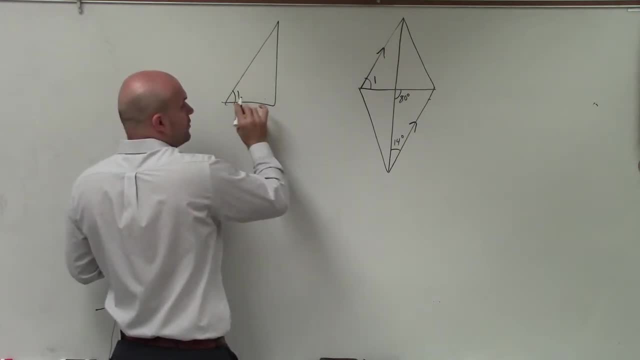 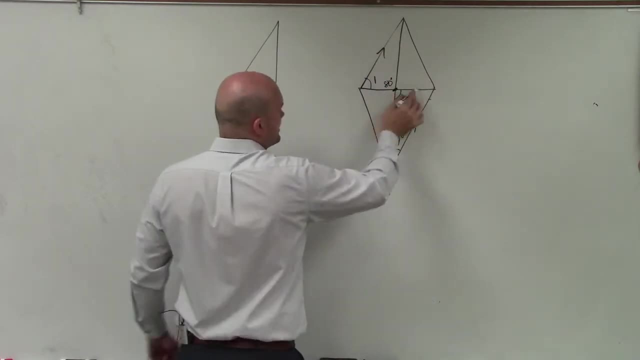 I want to figure out what these two are so I can figure out what angle 1 is. Well, notice that 80 degrees. I can apply my vertical angles right, Because they share a vertex but don't share any sides. So I can now say that that's 80 degrees. Now the last angle I need to figure. 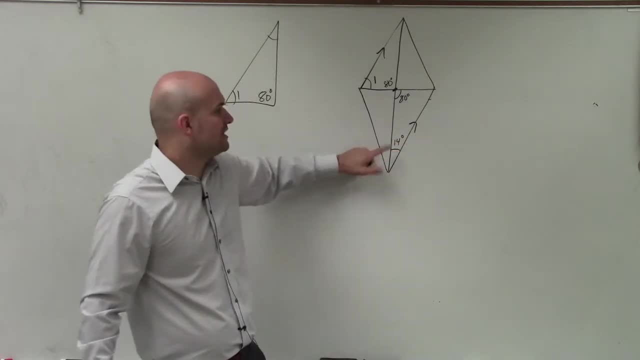 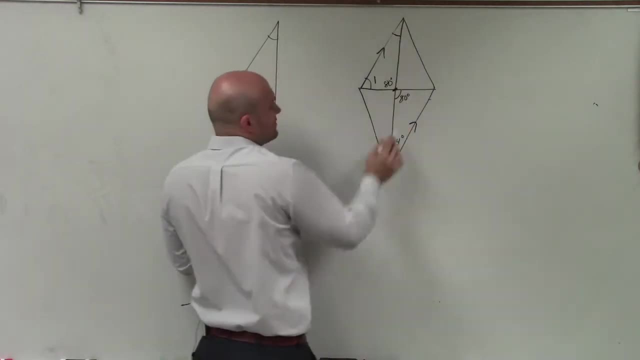 out is what is this one? And I know what 14 is, But how can I relate 14 to over here? Am I positive that those are the same? Well, I notice that 14 degrees and this angle are both on this line, right. 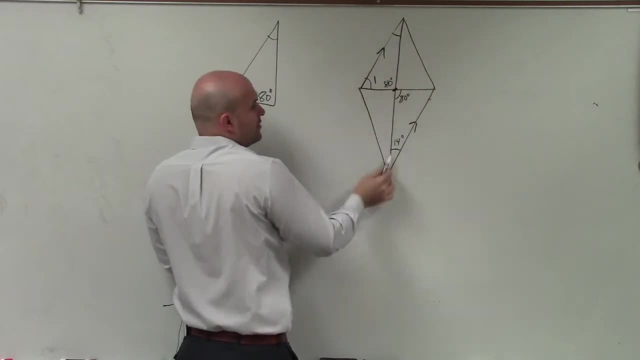 One is to the right, one is to the left. OK, They're both on this line and they both kind of touch our parallel lines. So what I'm going to do is I'm going to kind of forget about all of these lines for a second and see if I extend these parallel lines. what I have 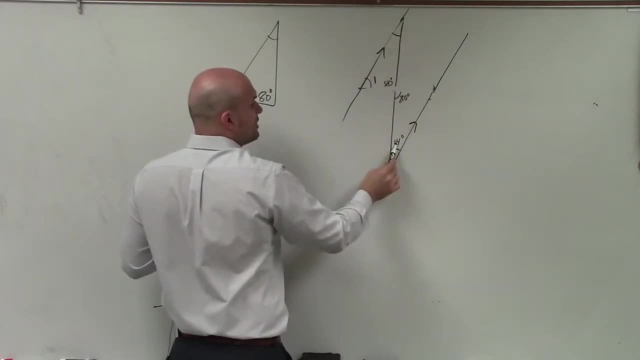 is yes. I have a relationship of parallel lines and a transversal where this is 14 degrees. That means this angle has to be 14 degrees by alternate interior angle. So I use my angle relationships, vertical angles as well as alternate interior angles. 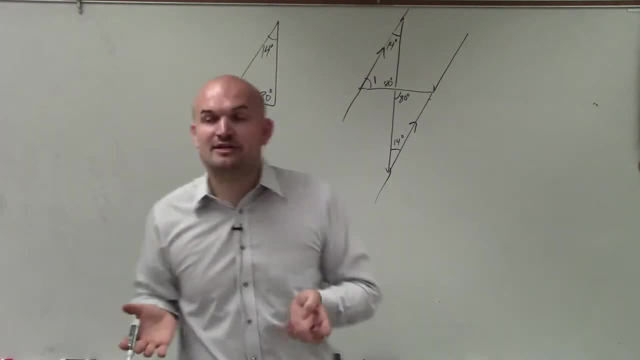 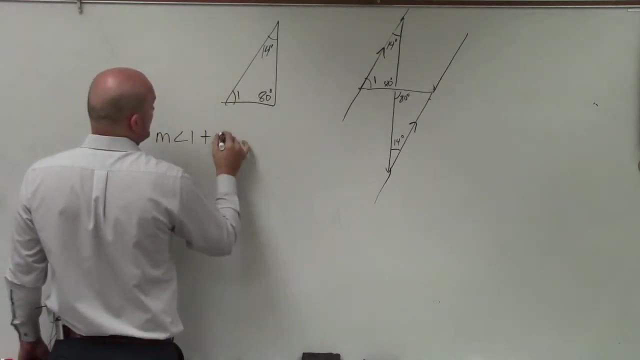 to find the measure of this angle Now, all I simply need to do is use the triangle sum theorem to be able to find my missing measure. So I'll create a formula. So measure of angle 1 plus 80 degrees plus 14 degrees. 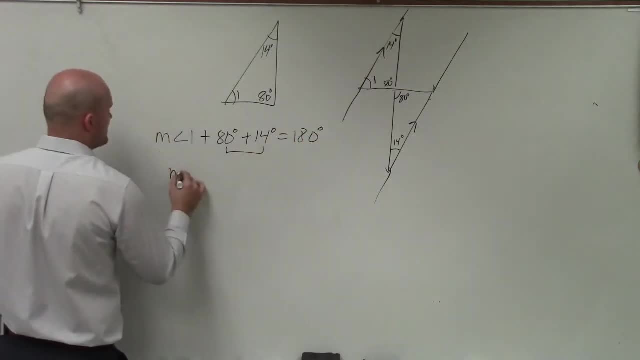 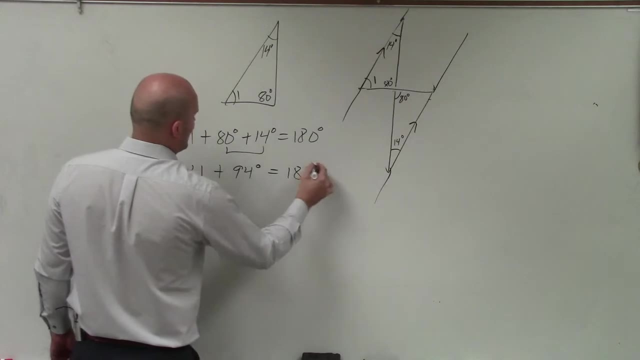 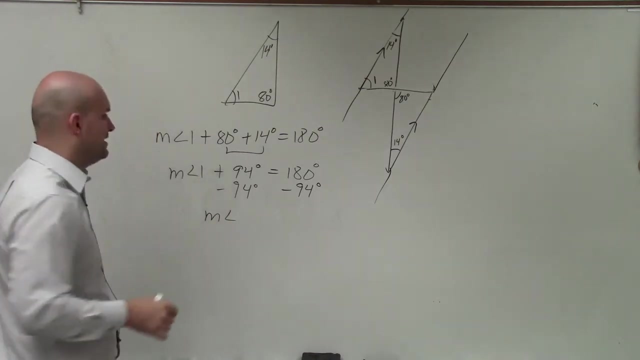 equals 180 degrees. Combine these, Measure of angle 1 is equal to 94,. oh sorry, measure of angle 1 plus 94 degrees equals 180 degrees. Subtract 94 degrees, Measure of 81 is going to equal 86..